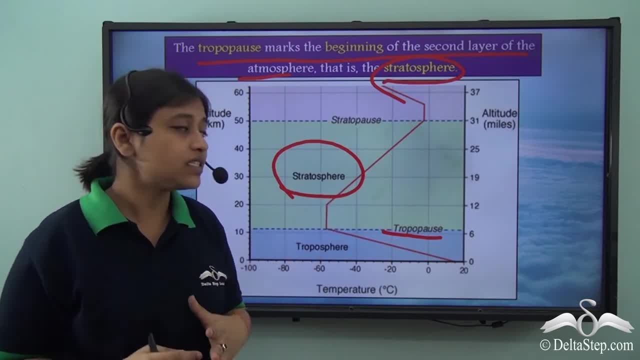 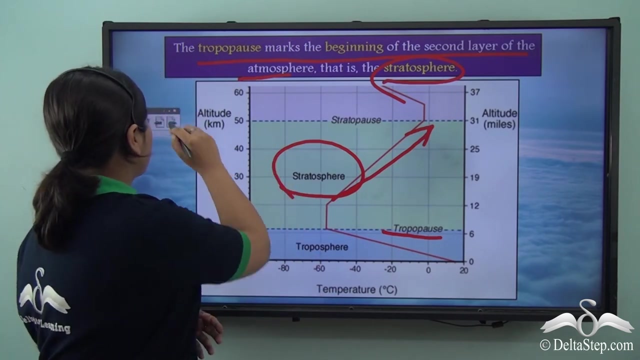 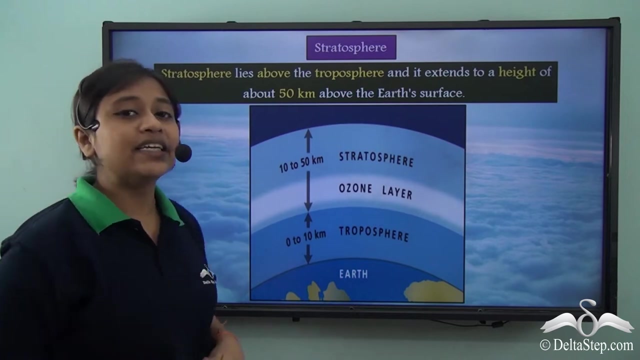 tropopause, where there is no mixing of temperatures in the stratosphere, what happens is the temperature starts gradually rising, right. So as we go higher into the stratosphere it gets hotter and hotter. So, talking about the second layer of the atmosphere, that is, stratosphere, it 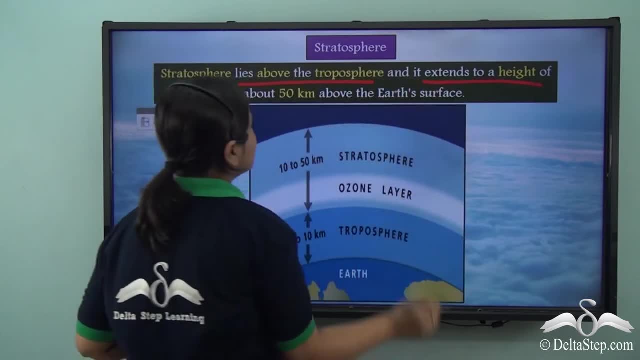 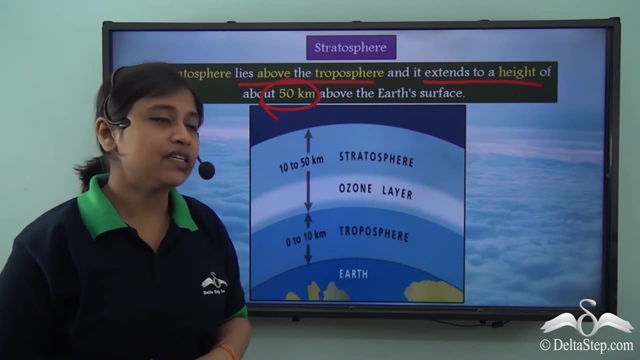 is above the troposphere and extends to a height of 50 kilometers from the earth's surface, as you can see here. We also need to remember that in this particular layer we have a very important region, and that is the ozone layer. We will learn about this later in details, but we need to remember that. 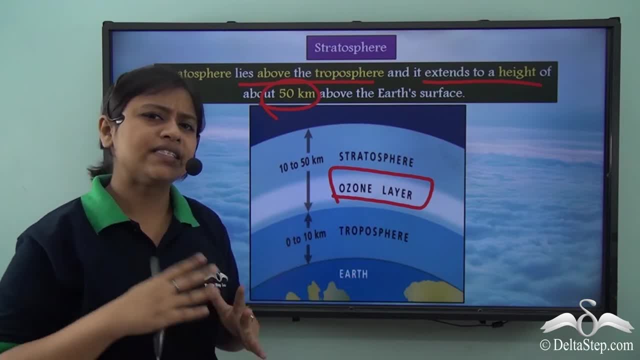 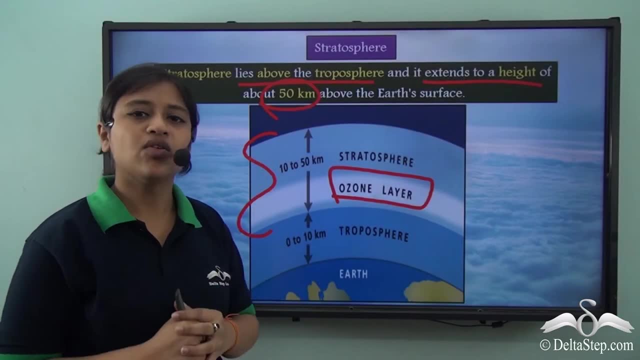 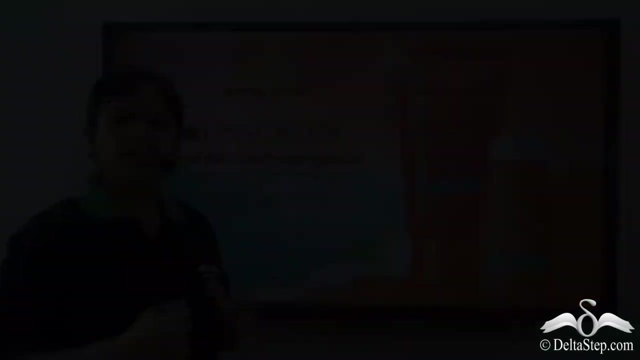 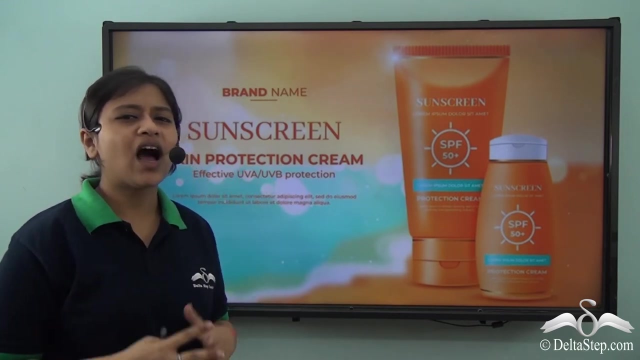 ozone layer is nothing different or separate part from this layer. it is just a part of this layer. So the stratosphere is inclusive of the ozone layer. So you must have seen various advertisement on different types of sunscreens. So what exactly do they do? They protect our skin from the harmful ultraviolet rays of the 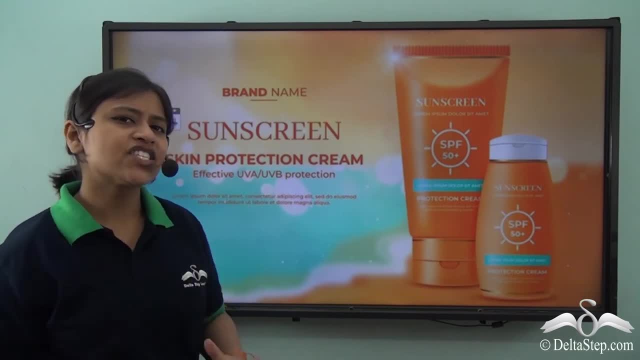 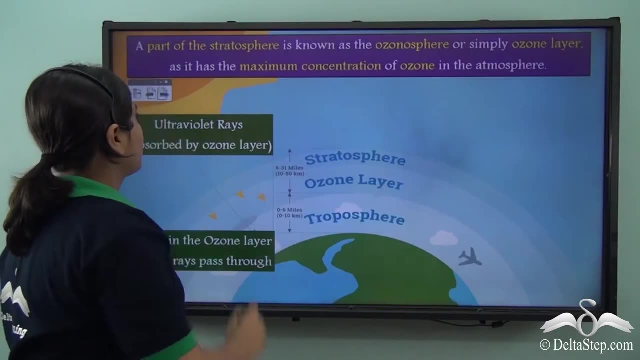 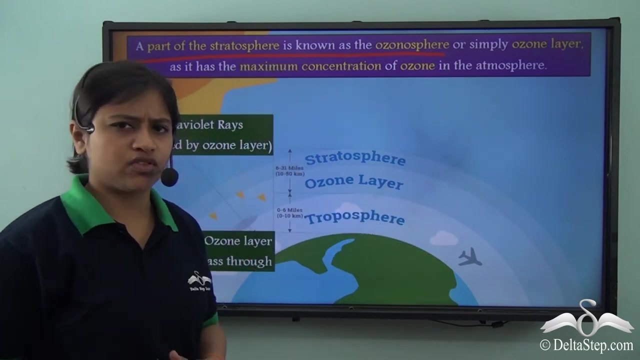 Sun, right, But there is a natural sunscreen that the earth also has. So even the earth has a sunscreen, And that is the ozone layer. So a part of the stratosphere is known as ozonosphere, or simply the ozone layer, and it has the maximum concentration of ozone in the 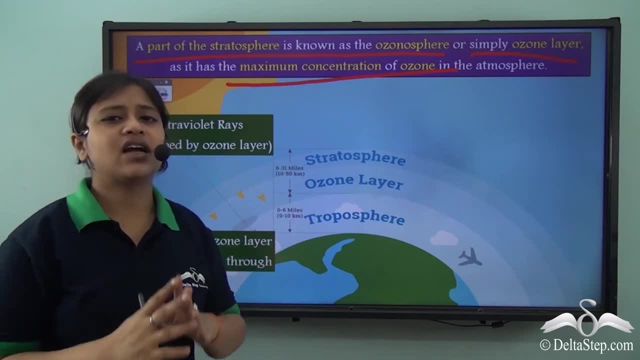 atmosphere. So, basically, ozone layer is nothing separate from this layer of atmosphere. It is just a part of stratosphere, right? There is high concentration of ozone in the lower region of this stratosphere. Now what does it do? This ozone layer acts as a sunscreen, as I've 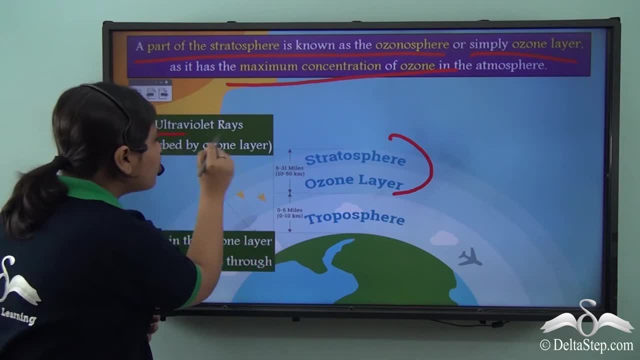 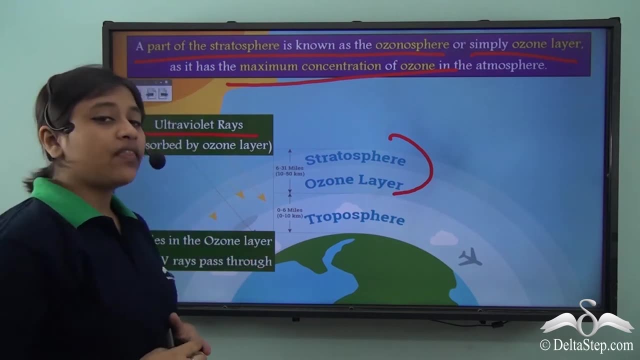 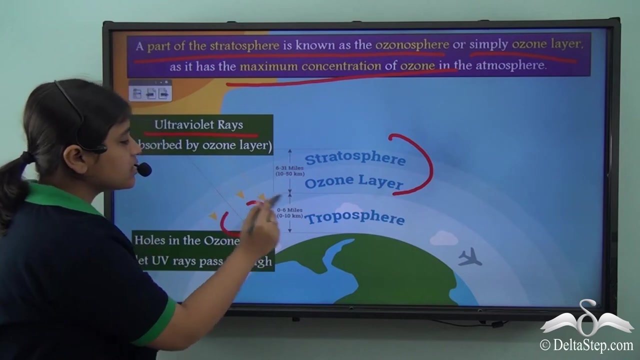 already mentioned, It absorbs the harmful ultraviolet rays of the sun. that could cause major damage to our health and skin And there is a problem. What is the problem? Due to various human activities, there are holes in this ozone layer that has occurred over the years. So these holes in the ozone layer are…. 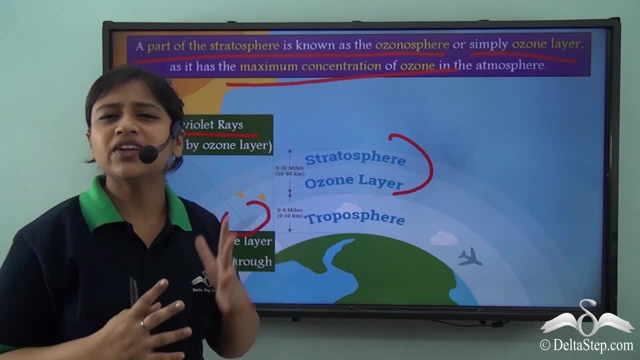 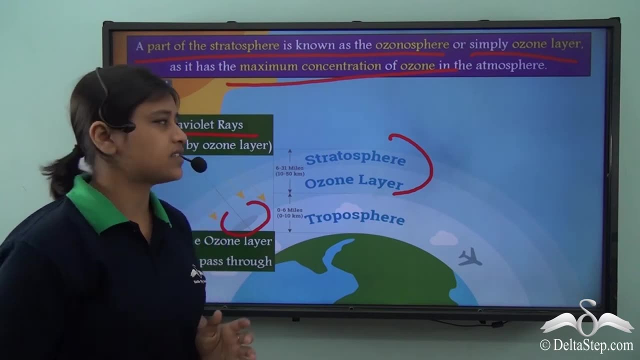 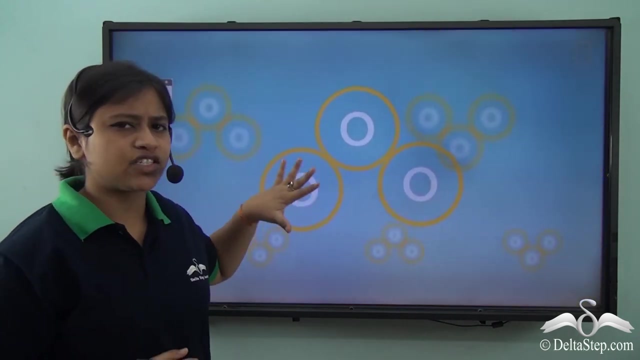 layer are letting or allowing the UV rays, the harmful UV rays of the Sun, to reach the Earth's surface directly, which is not very right. So let's see a video on this, So you see that the ozone layer is a part of the stratosphere with high 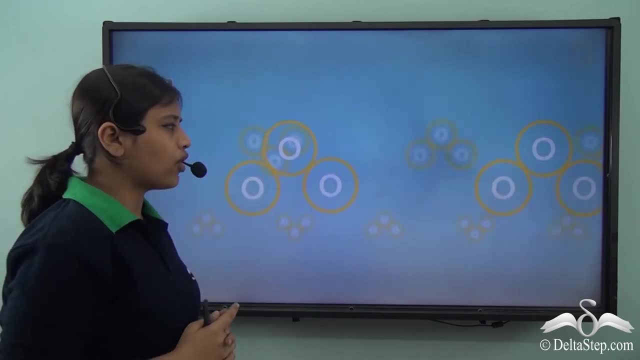 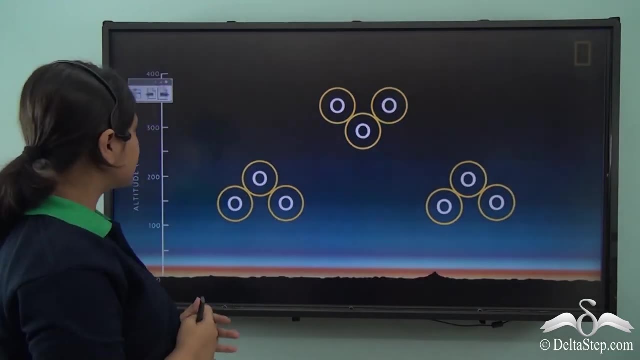 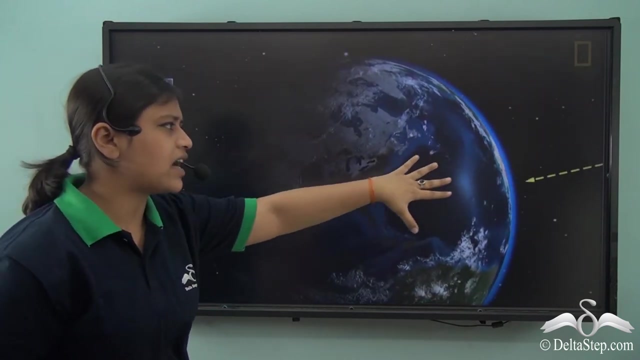 concentration of ozone gases here. So what do they do? They are here to protect the Earth from the harmful ultraviolet rays. So you can see they are present at this altitude where they protect the Earth from the harmful ultraviolet rays that could directly pass through the atmosphere. So they filter these. ultraviolet rays and radiate it back into the space. Coming to another very interesting fact, Well, do you know why is it convenient to fly airplanes and commercial jet aircrafts in this layer of the atmosphere? Well, this is because of the absence of clouds and very little water vapor and dust particles present. 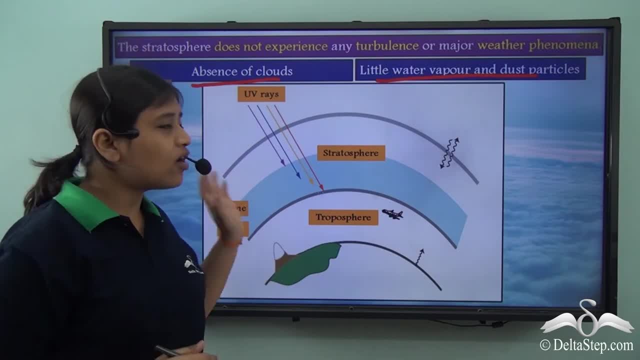 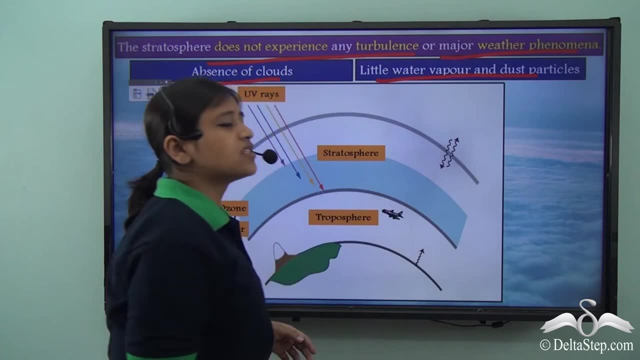 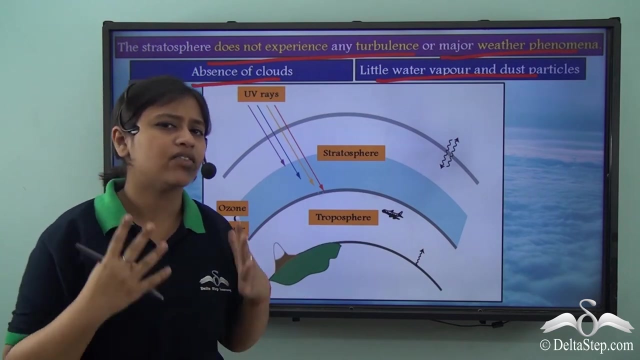 in this particular layer of the atmosphere. So because of this, it experiences no turbulence and weather phenomena does not occur at this part of the atmosphere. It generally occurs in the first layer of the atmosphere, as we have learnt in the last video, right? So you? 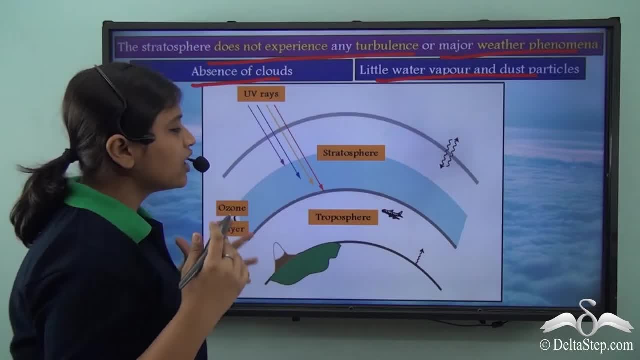 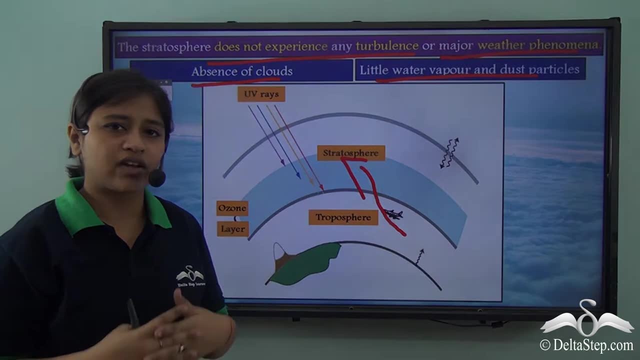 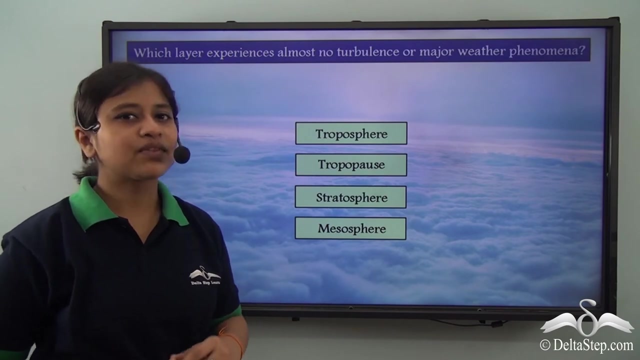 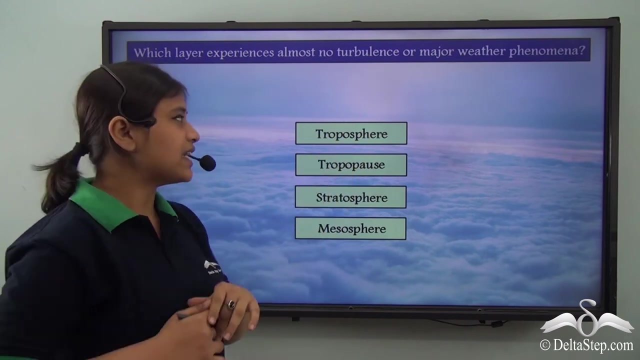 see that the planes, the commercial plane and jets. they usually climb to the second layer of the atmosphere, where there is no turbulence due to the absence of clouds, and it can easily travel. So can you help me answer this question? Well, which layer experiences almost no turbulence or major weather phenomena Is? it troposphere? is it tropopause or stratosphere? or is it the mesosphere? Yes, the answer is the stratosphere, due to the absence of clouds and very little dust particles and water vapor. Now, just like tropopause is the boundary of the first layer of the atmosphere. Similarly, stratopause is the boundary of the atmosphere, boundary or the end of the second layer of the atmosphere, and that is stratosphere. So now let's summarize the second layer of the atmosphere. So the very first point says that it extends up to 50 km from the earth's surface. 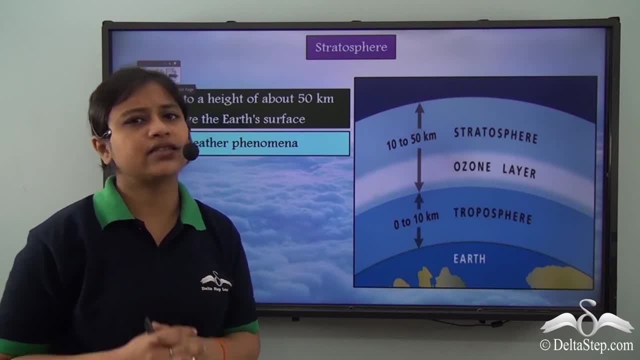 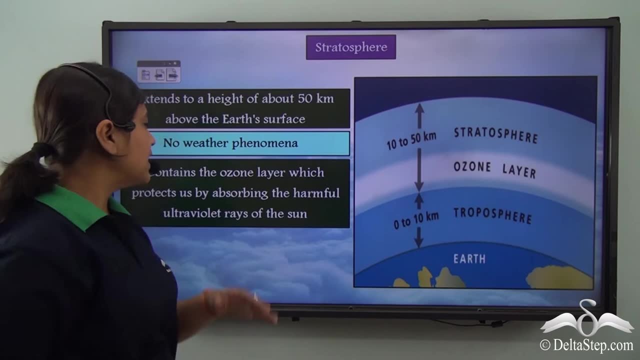 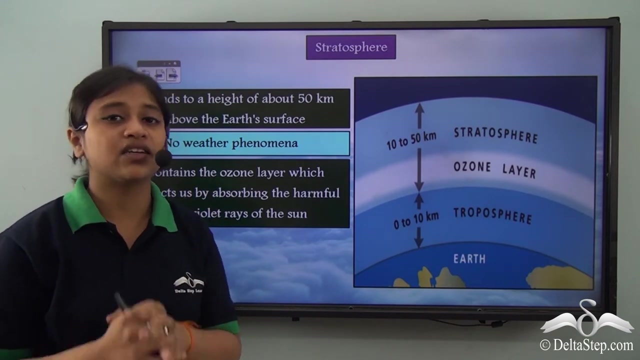 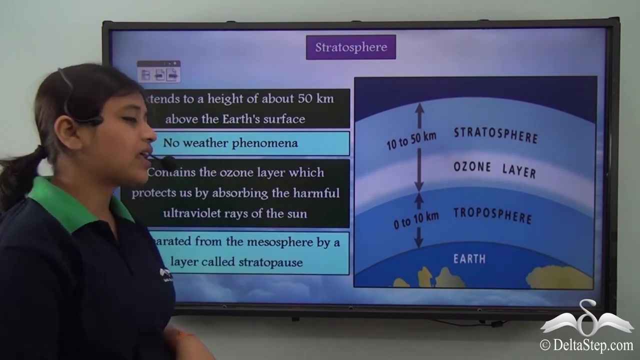 Next, due to absence of clouds and very little dust particles and water vapour, there is no weather phenomena. Also, it contains the ozone layer, which protects us from the ultraviolet rays of the sun that are very, very harmful, thus acting as a very good sunscreen. 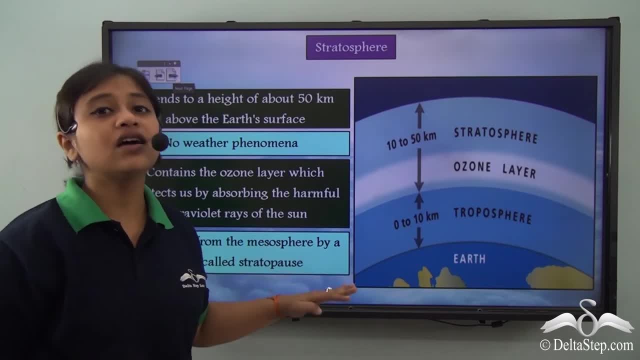 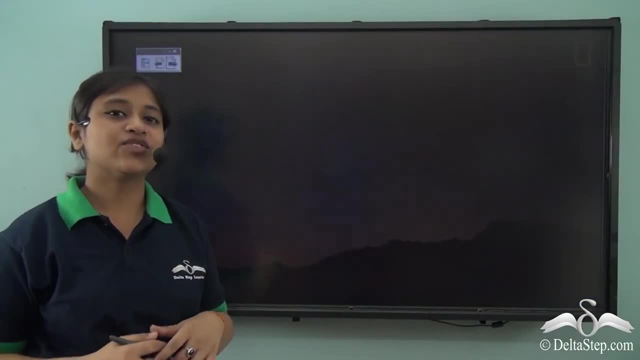 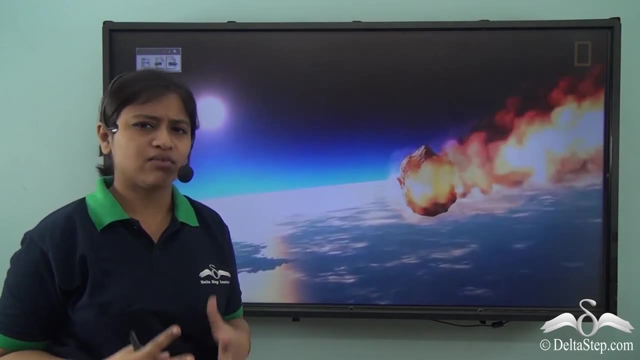 Lastly, it is separated from the mesosphere, that is, the third layer of the atmosphere, by the stratopause Right. So now we will study about the third layer of the atmosphere, that is, the mesosphere. So we know that the earth's atmosphere protects us from meteorite encounters. 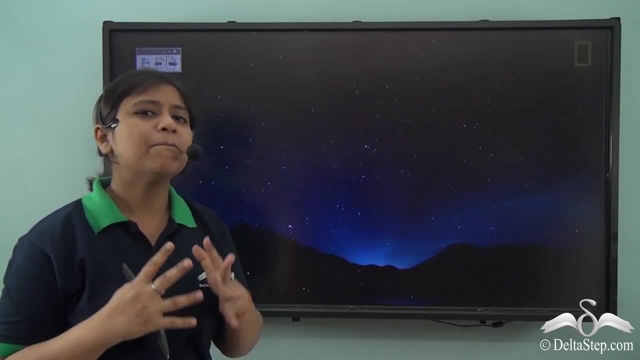 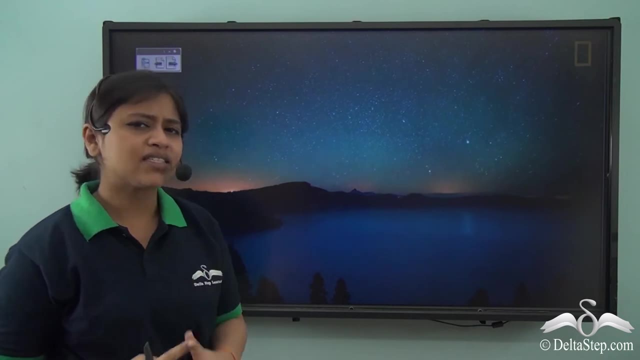 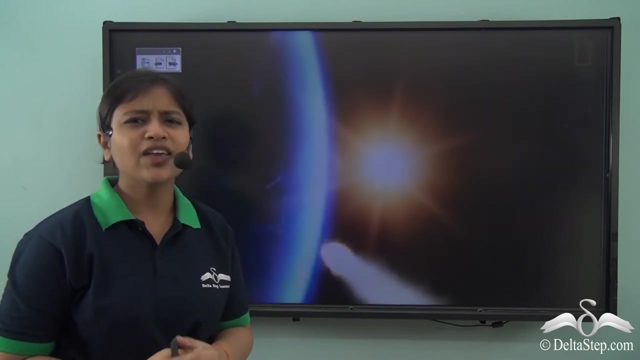 This is actually done by this layer of the atmosphere. The mesosphere does not let the meteorites come into the atmospheric layers, So it protects the earth. These meteorites, on entering the atmospheric layer, turns into meteors or shooting stars. You must understand this. You must have heard about shooting stars, Aren't they very beautiful? Well, this is all because of these meteors that enter into the earth's atmosphere. Therefore, the mesosphere lies just above the stratosphere and it is separated by the stratopause. Stratopause, that is, the end of stratosphere, also marks the beginning of the mesosphere. Now, The word mesosphere is derived from the Greek words mesos and sphira. So what does this mean? This means middle layer. So we now know that mesosphere is the middle layer of the atmosphere. 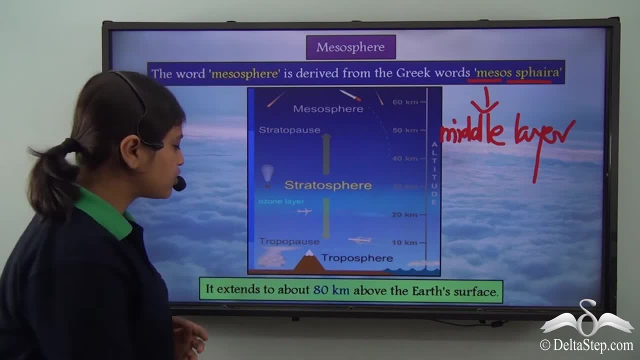 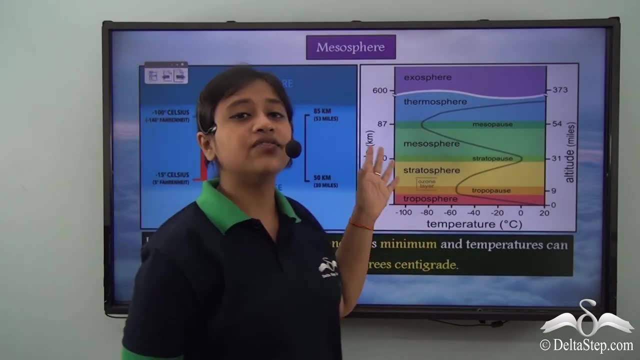 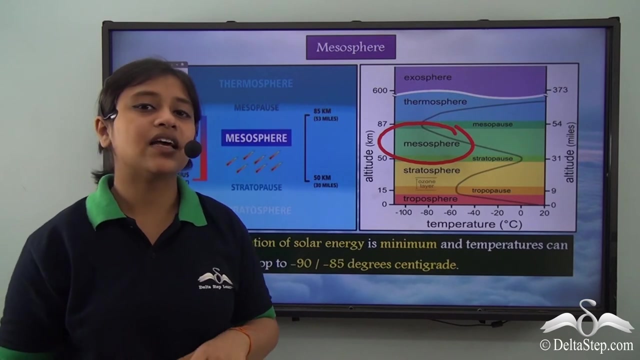 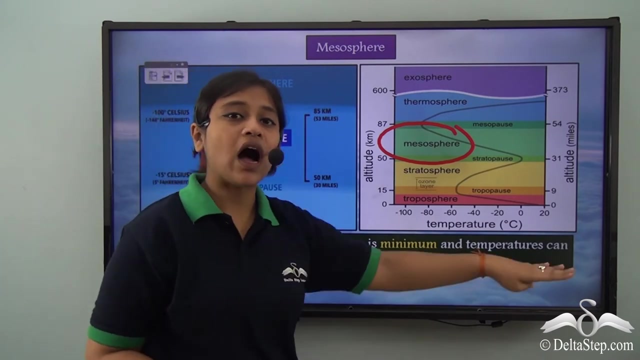 Right, And also it extends up to 80 kilometers from the earth's surface. So, As you can see On this very graph, that mesosphere lies just in between the atmospheric layers. thus it is known as the middle layer of the atmosphere. Now we have learnt that as we go higher in the tropospheric layer, the temperature falls. 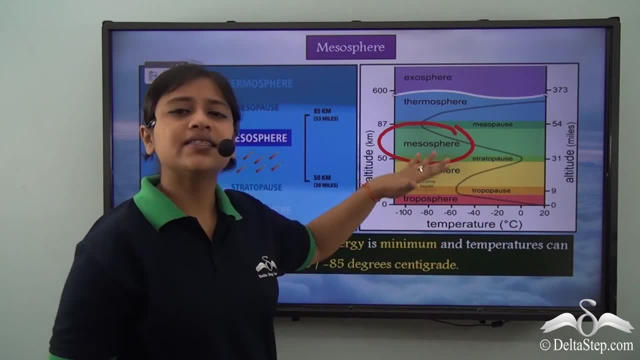 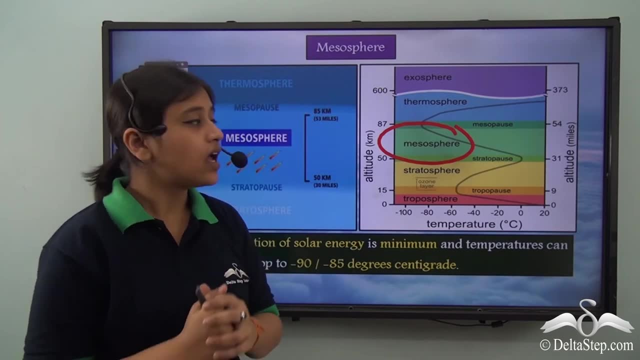 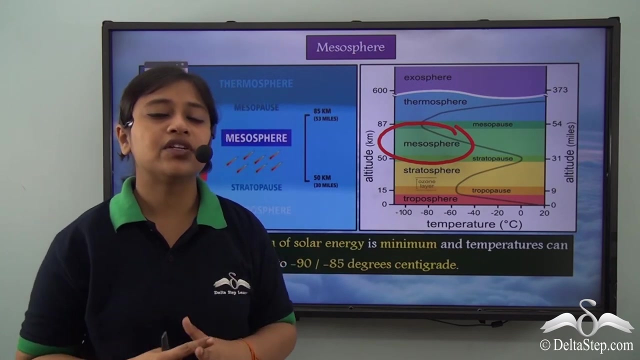 down, So it gets cooler While we enter the second layer, that is, the stratosphere. it gets hotter as we go higher into the stratospheric layer. Now, when we come into the mesosphere or the third layer of the atmosphere, what happens is the temperature starts falling rapidly because of the minimum absorption of solar 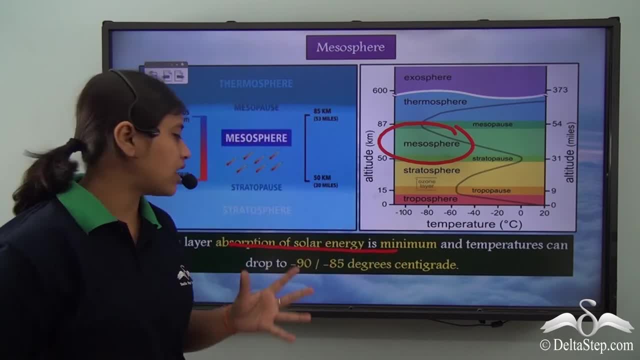 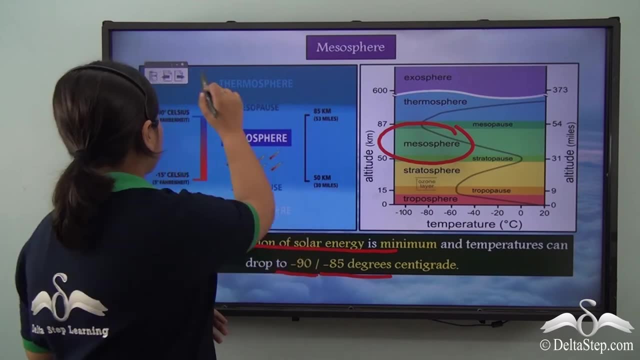 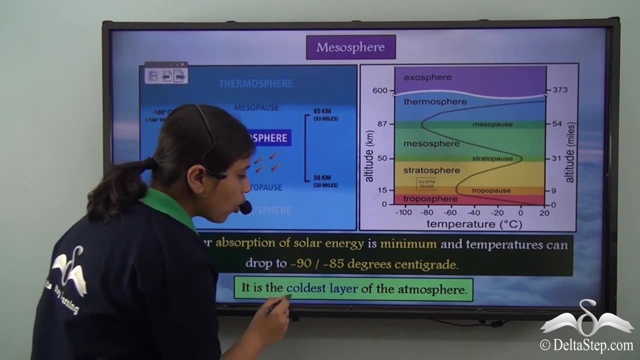 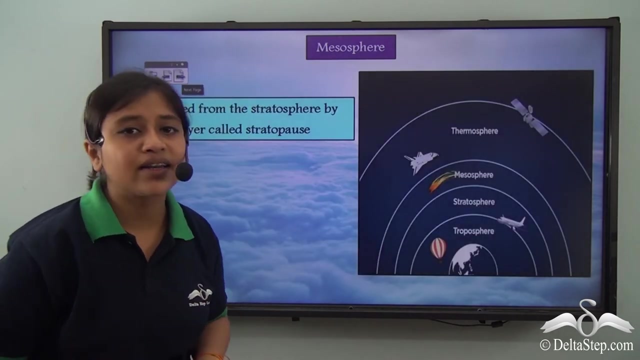 energy in this layer. So the temperatures can fall down up to minus 90 degree or minus 85 degree centigrade. So because the temperatures fall down to that very extent, it is known as the coldest layer of the atmosphere. So let's summarize: the third layer of the 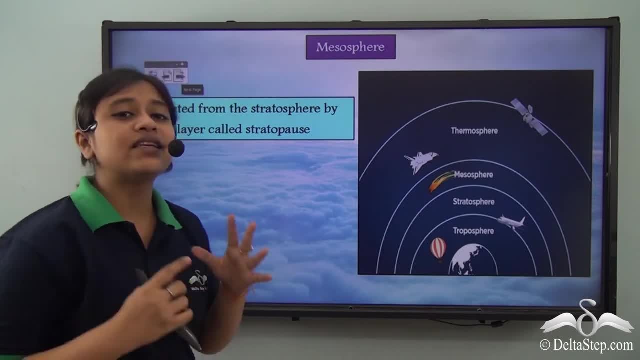 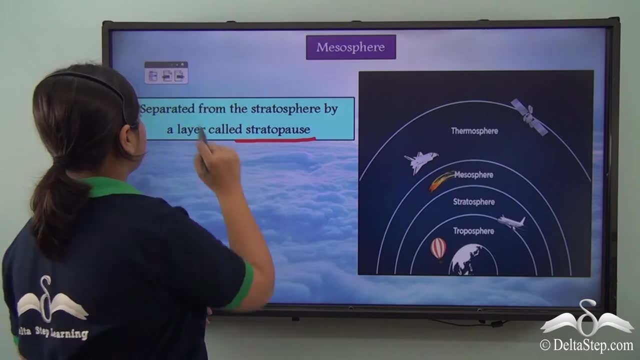 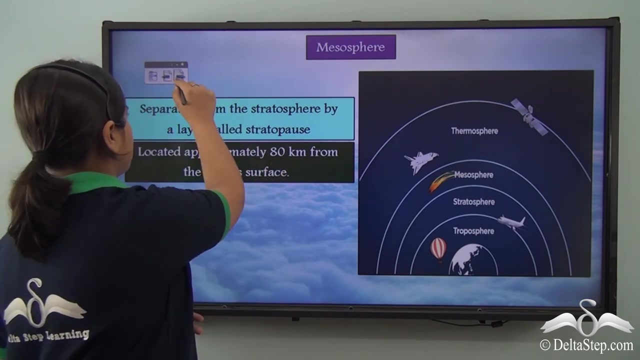 atmosphere. The very first point says that it is separated from the stratosphere with this layer, the stratopause. Secondly, it is located approximately 80 kilometers from the earth's surface. Thirdly, meteors burn in this layer due to friction. And lastly, 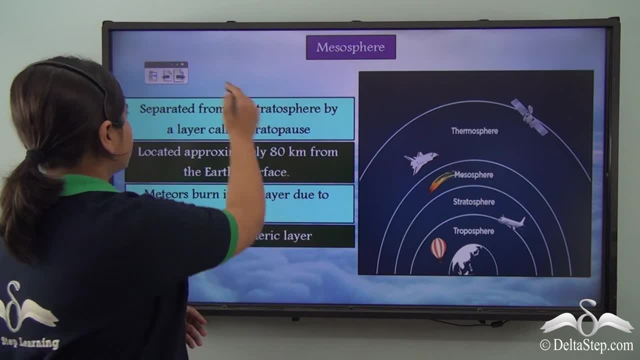 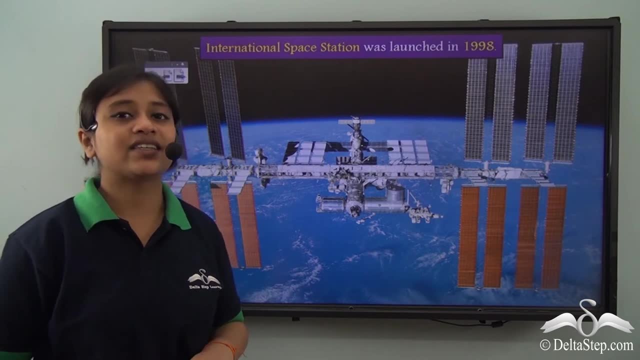 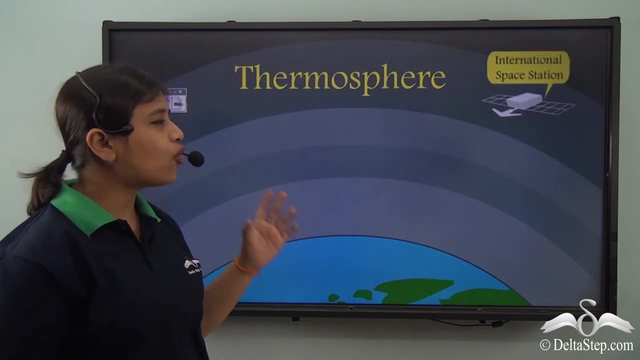 it is the coldest layer of the atmosphere. So what do you see here? Well, this is the International Space Station that has been orbiting since its launch in 1998.. So where is this located? 1. So the International Space Station is located in the fourth layer of the atmosphere, and 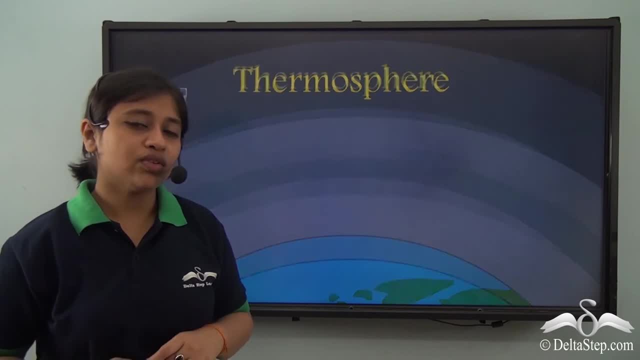 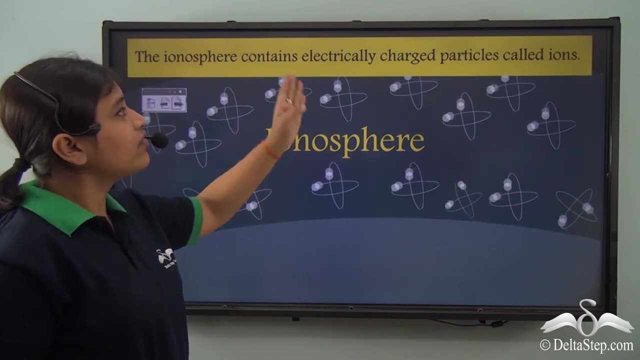 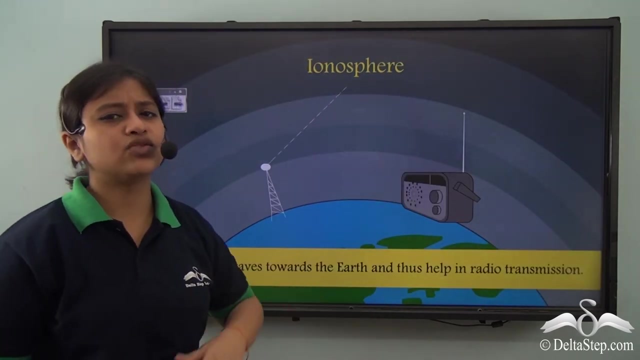 that is the thermosphere. You also need to know that the thermosphere is also known as ionosphere. Why is it so? Because of the presence of electrically charged particles called ions. These ions reflect radio waves to the earth's surface and help in radio transmission. So 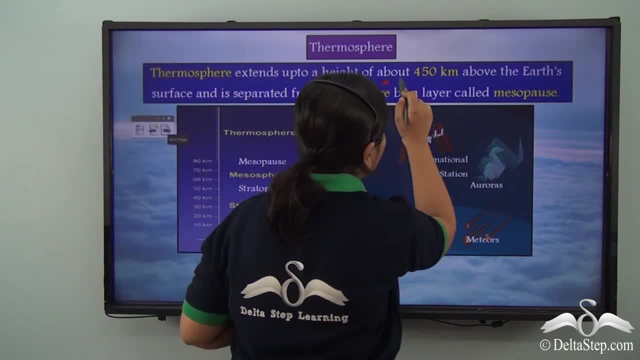 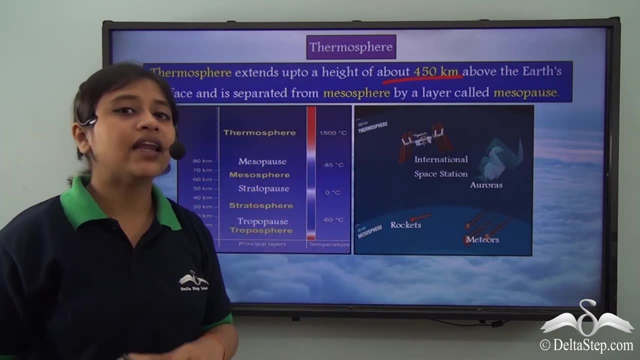 in this solar intense atmosphere. When a thermosphere hits the earth, it will heat up, butterup places. So see, that's the thermosphere where, that's the thermosphere. Let's see what happened in the third layer. So in the third layer, first and foremost, 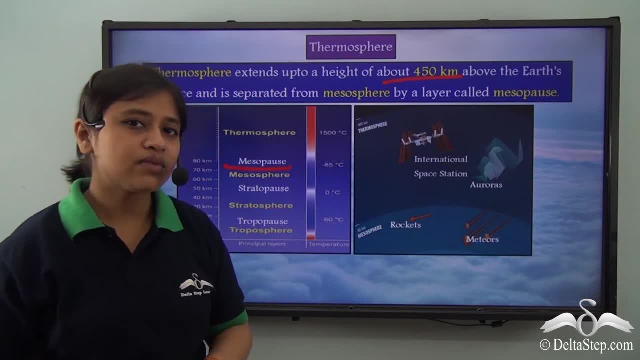 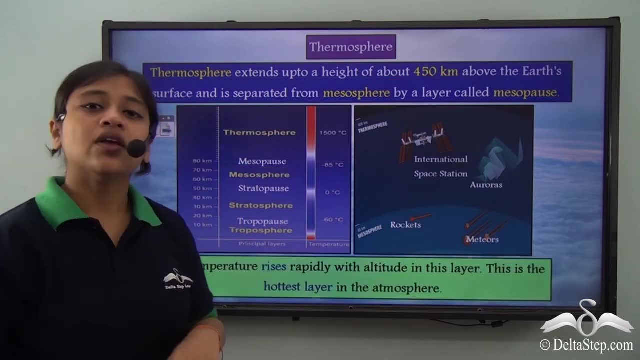 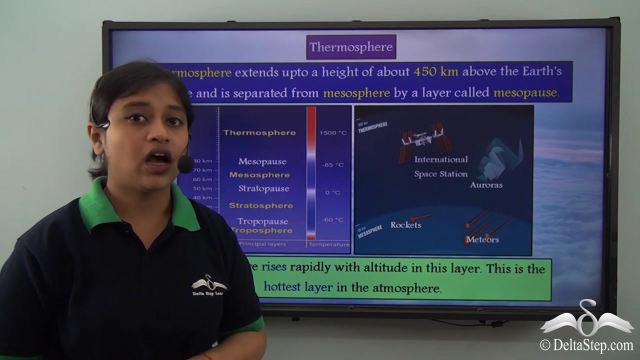 it is separated from the stratosphere by the layer called the Mesopause. So the mesopause, while it marks the end of mesosphere, at the same time it also marks the beginning of the thermosphere Right. 2. the coldest region or the coldest layer of the atmosphere. On the other hand, the layer just above it, that is, thermosphere, is the hottest layer of the atmosphere. Why so? Because the temperature starts rising rapidly with the altitude in this layer. So from the very word thermo, which is related to heat, we know that this is the hottest layer of the atmosphere. 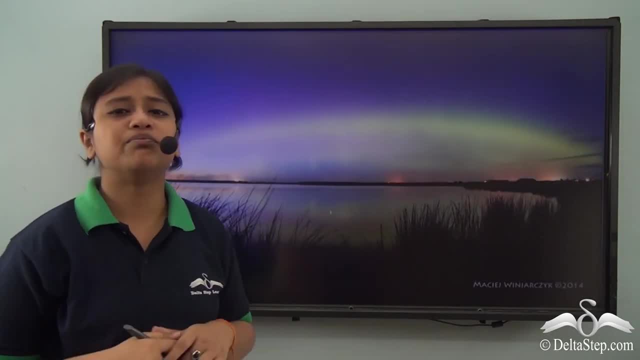 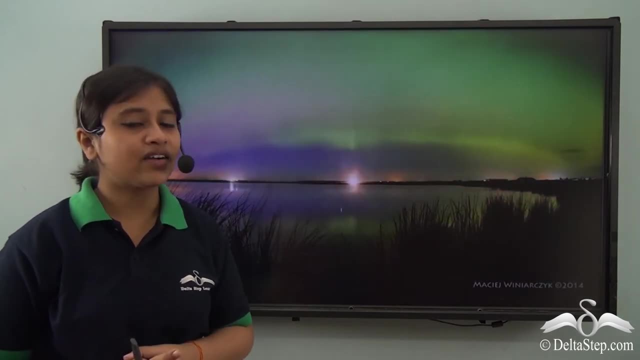 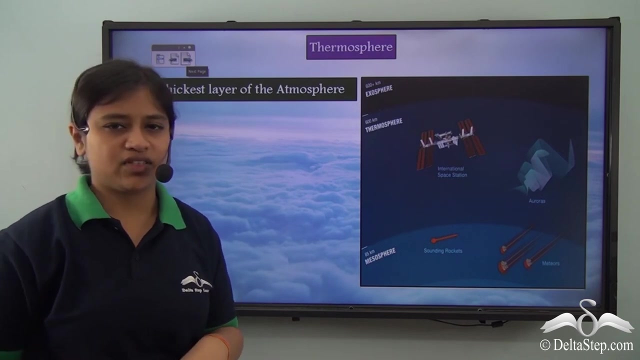 Now have you heard about this beautiful phenomena? This is Aurora. that is usually seen in the polar regions and tends to occur in the thermosphere. So now let's summarise the fourth layer of the atmosphere. The very first point says that it is the thickest layer of the snel. 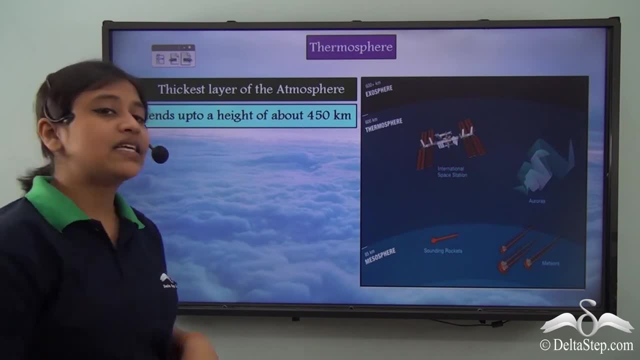 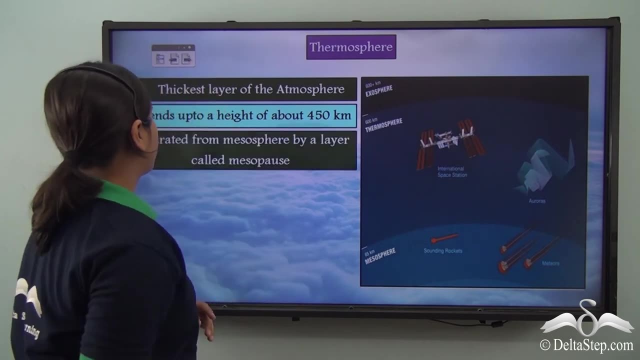 atmosphere Right? Secondly, It extends up to 450 degree kilometer from the earth's surface. Thirdly, it is separated from the mesosphere by the mesopause layer. So now, how do you remember which is the hottest layer of the atmosphere? 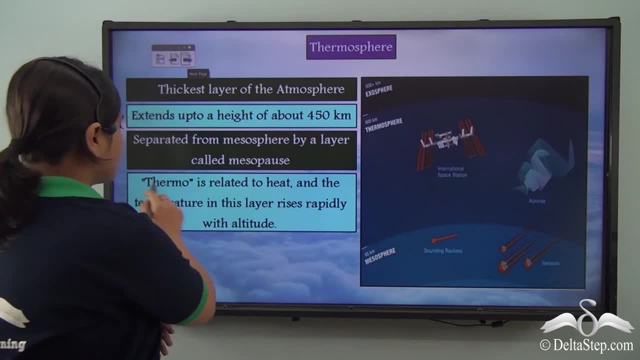 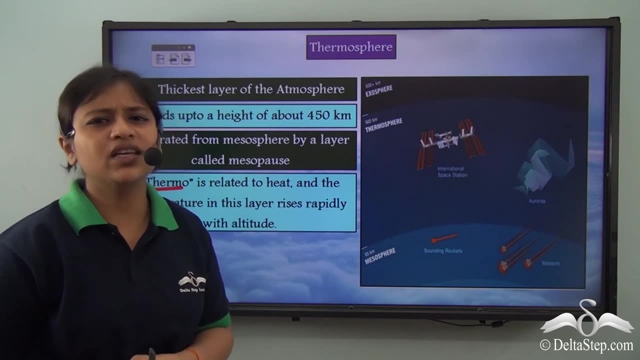 Well, the very name thermosphere, out of which thermo is related to heat. So it is very simple that this layer is the hottest layer of the atmosphere. Well, the obvious reason is also that the temperatures rise very rapidly with altitude in this layer. Lastly, it facilitates. 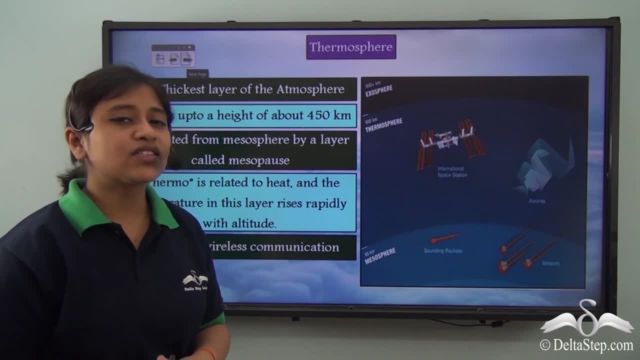 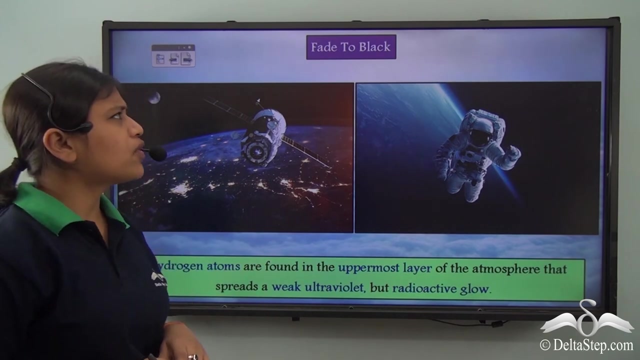 wireless communication. Why so? Because of the presence of electrically charged ions. that reflects radio waves back to the earth's surface and help in radio transmission. We must not forget of the beautiful phenomena, Aurora, that also occurs in this layer. Now, so what do you understand from the title? Fade to black, Interesting right. Well, here. 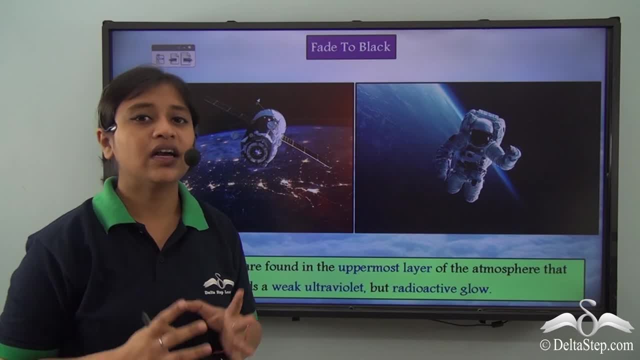 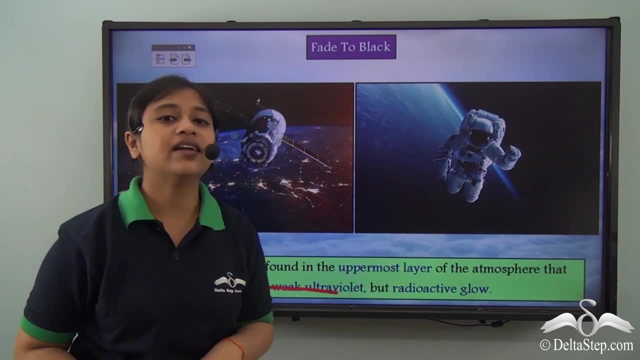 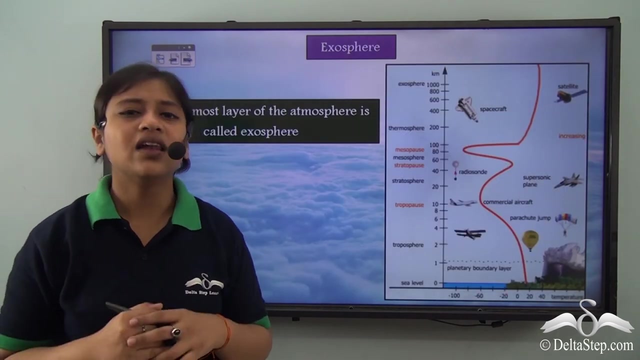 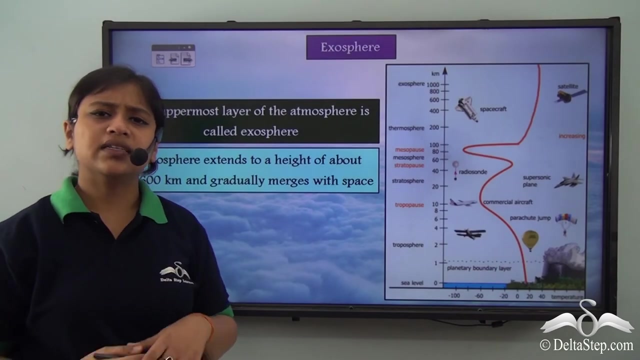 we are talking about the uppermost layer of the atmosphere. Here there is presence of hydrogen atoms that spreads weak ultraviolet but radioactive glow. So this is the uppermost or the last layer of the atmosphere. It is known as exosphere. right Now it is believed that exosphere extends up to a. 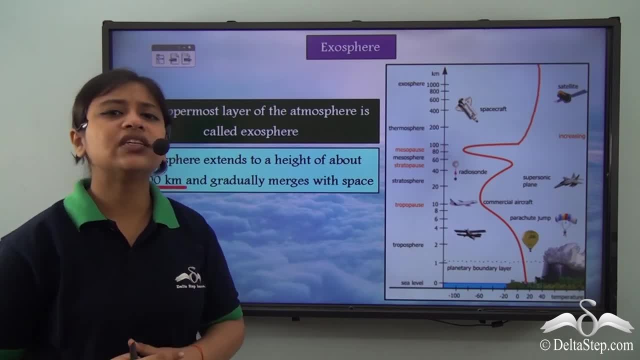 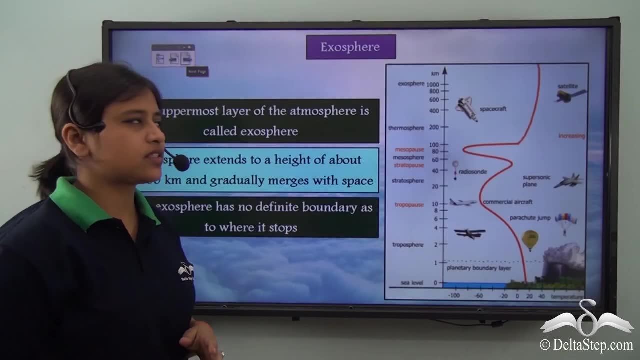 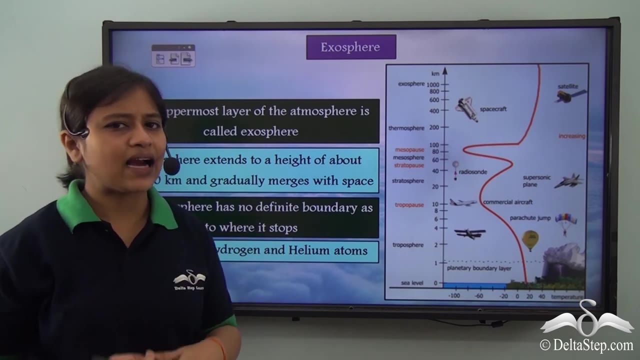 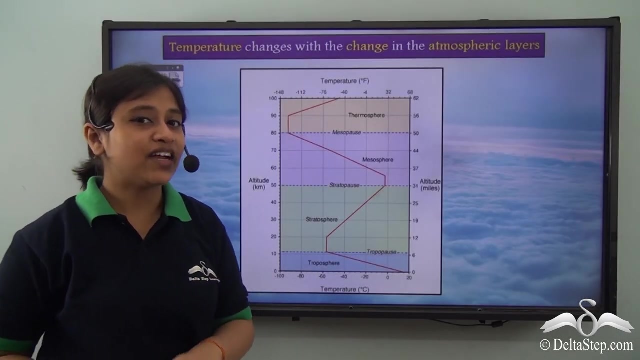 height of 1600 km and gradually merges with this space. Therefore, there is no definite boundary as to where this layer stops. Lastly, we also know that there is presence of hydrogen and helium atoms in this particular layer of atmosphere. So if you have been very attentive, you must have noticed that the temperature fluctuation 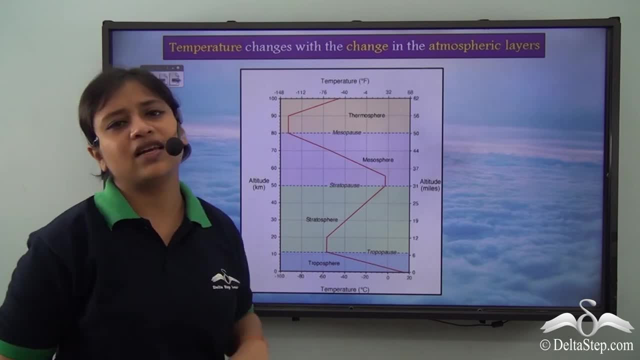 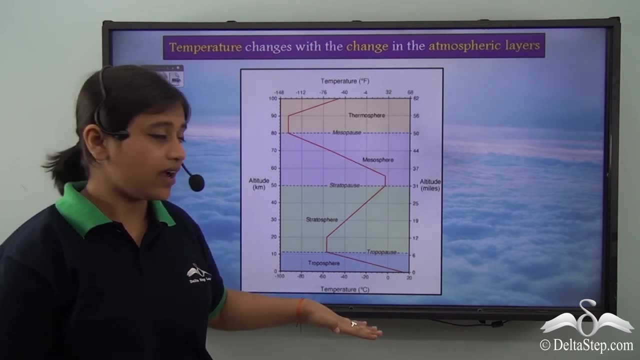 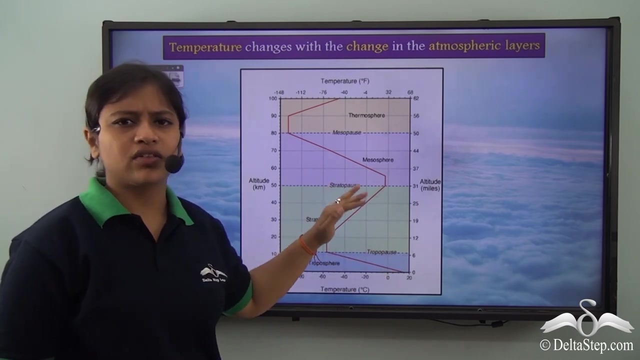 in the different layers of the atmosphere is almost in a zig-zag pattern. So in the first layer the temperature falls as we go higher in this layer, while in the second layer, on going higher, we see that the temperature is rising Again in the mesosphere or the 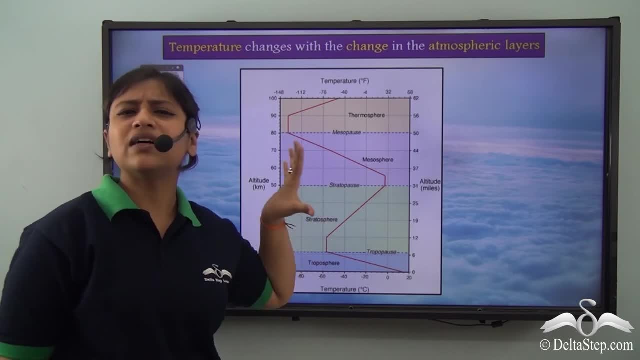 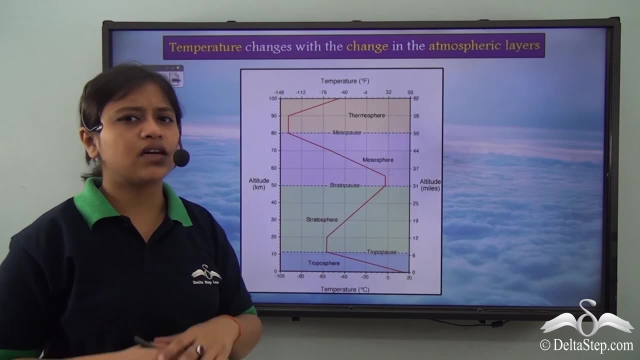 third layer, we see that the temperatures are falling to a great extent, So we are making it the coldest layer of the atmosphere. Again, going to the fourth layer, that is thermosphere, the temperatures rise up to a great extent and makes it the hottest layer of the atmosphere. 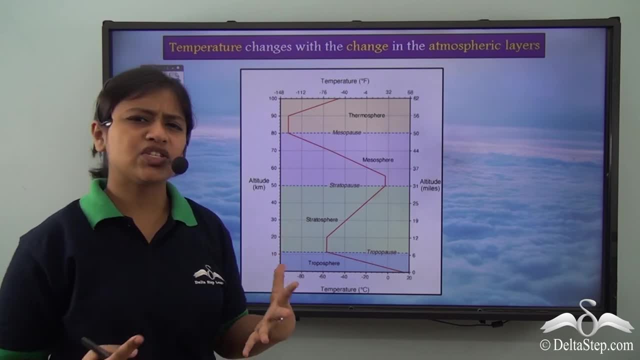 So we don't really have much information about the temperature changes in the last layer or the uppermost layer of the atmosphere, that is, exosphere, because research is still going on about this layer. Not much is known of this layer and scientists are still working on it, So let's move on to the next layer, which is exosphere. So